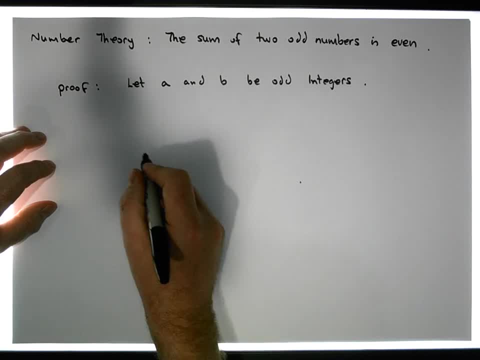 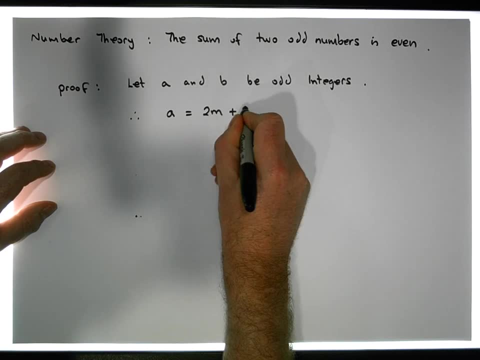 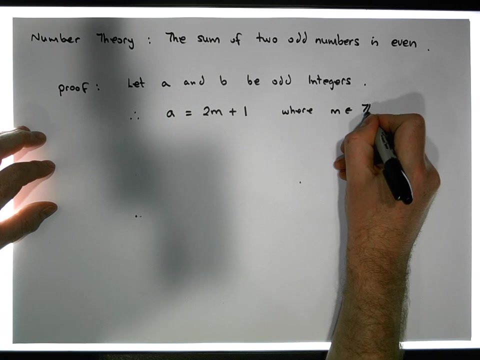 something like this: okay, So knowing that these two numbers are odd numbers, well then, based off the division algorithm. so therefore we have: A must be equal to two times some number plus one. okay, where this some number, M, is an element of the integer. 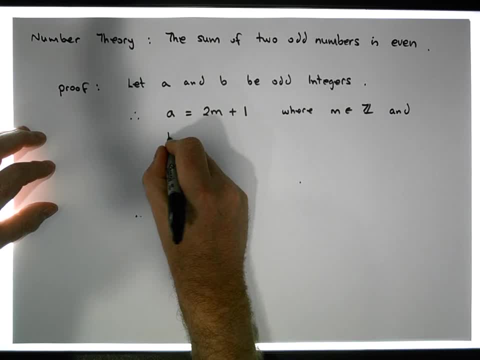 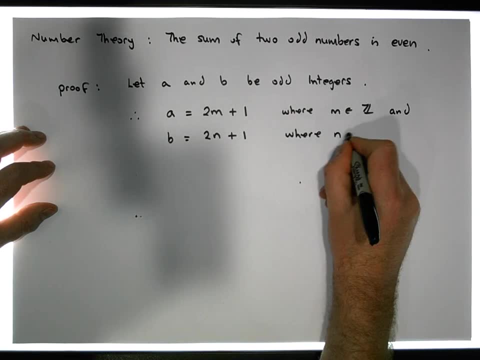 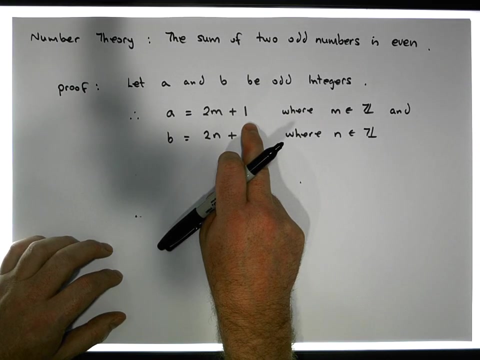 And also we must have that B must be equal to two times some other number, plus one where N is also an element of the integers. And this is just a fact. okay, based off the definition of even and odd numbers. okay, If the number was even, well, then when we divide in by two, there would be no. 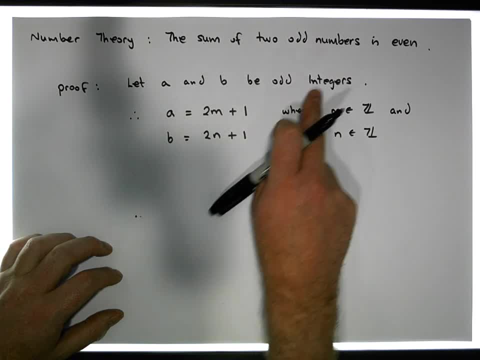 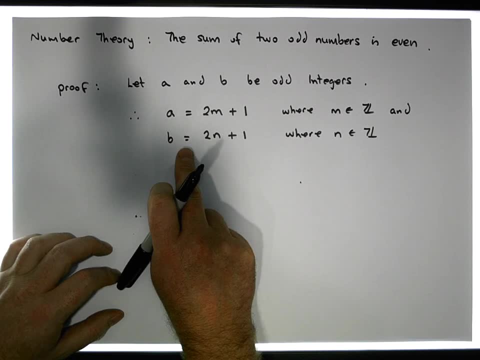 remainder. okay. So we've said that we need to have two odd numbers, so them odd numbers must look something like this: They must look like two times some number plus one. So if we divide in by two, they must look like two times some other possible number plus one. okay, So what does this? 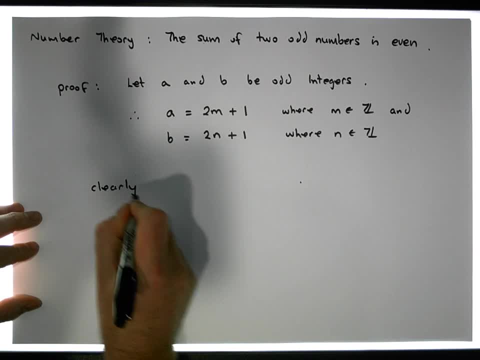 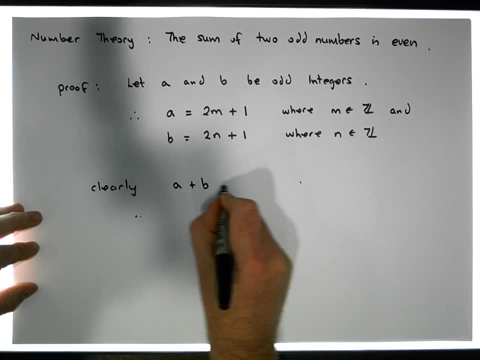 tell us: Well, clearly, we have something like this: now, okay, Let's add them together, because what we want to show is we want to show that the sum of these two numbers is even. So let's add them together. Well, A plus B is going to be equal to. well, A, by definition, is equal to two M. 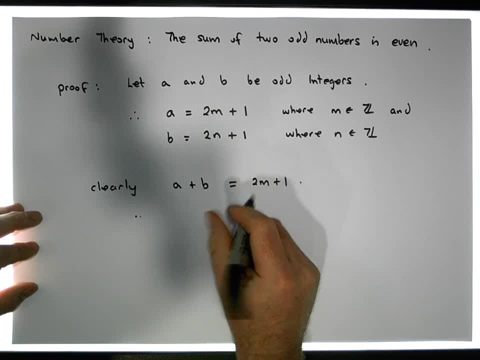 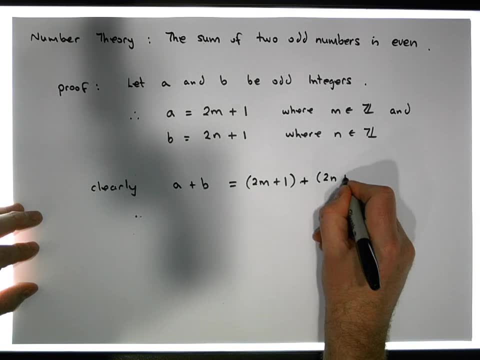 it's odd, two M plus one, okay, Plus okay, that's our A plus our B, which is, by definition, here it's odd, which it must be equal to two N plus one. So when we remove the brackets, what does that give us? That gives us two M plus one, plus two N plus one, okay. 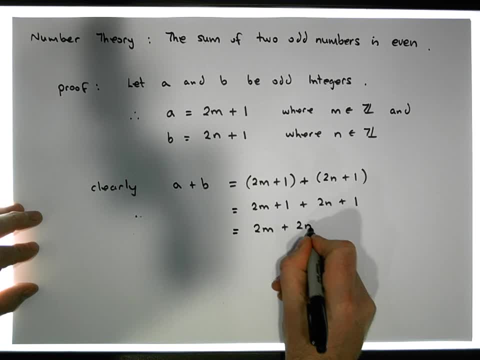 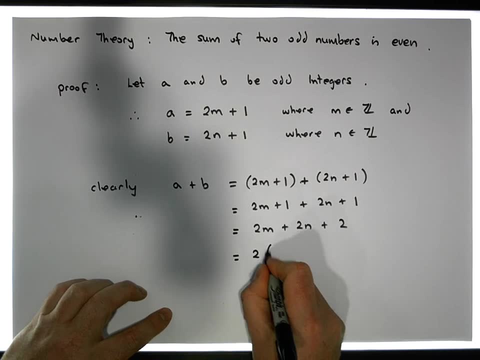 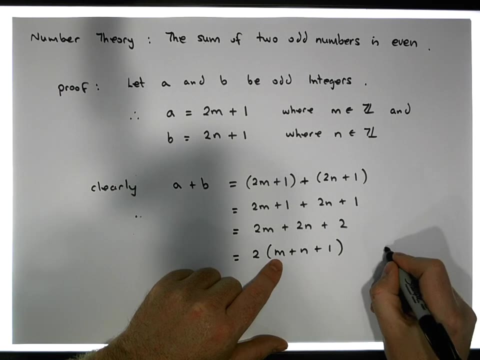 which is the same as two M plus two, N plus two. okay, Now, there's a common factor across here: it's two. So this is equal to two times M plus N plus one. okay, Now, clearly, M and N. M and N. 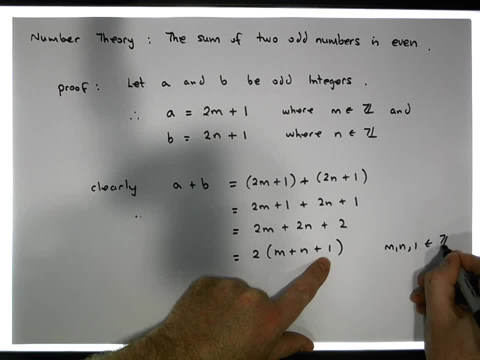 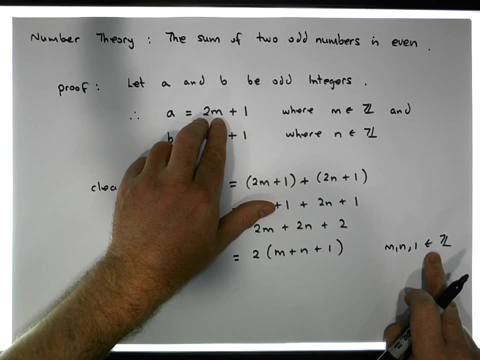 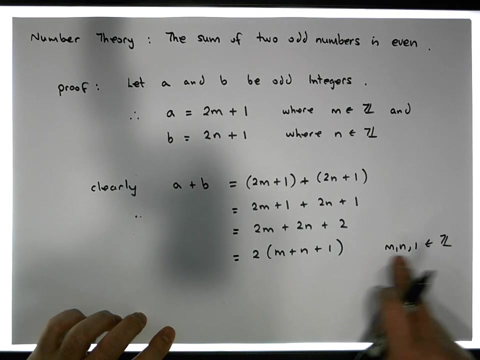 and also one okay are integers okay because we defined them earlier on to be integers okay, and that's a fact from the division algorithm. okay, that we can find two integers okay and a possible remainder okay. So when we add three integers together, we always get an integer.